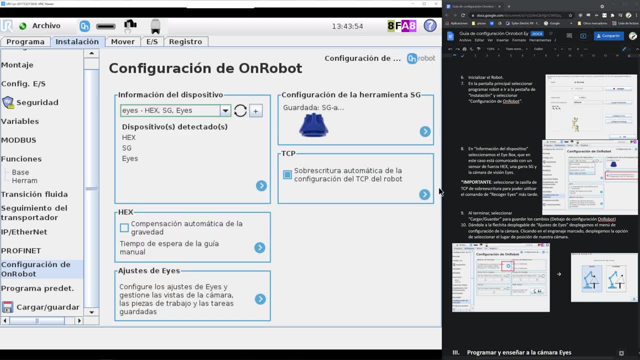 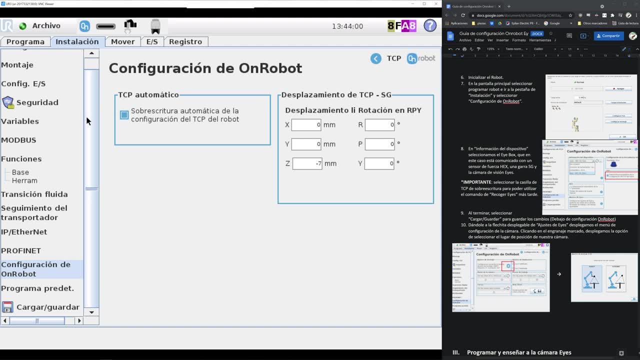 In addition you can also add working spaces and works. but we will do that directly in the L program. We double check that the TCP auto is enabled And we go into the configuration for TCP it's enabled. so now we go back to the program. 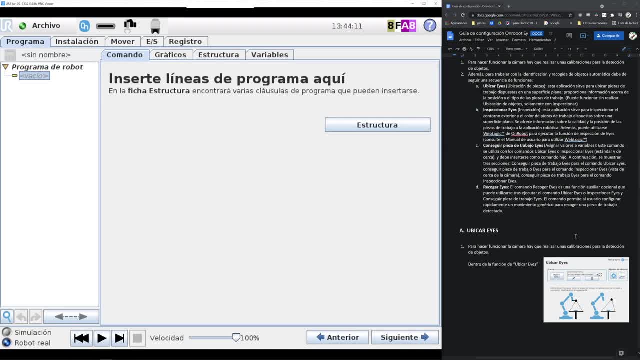 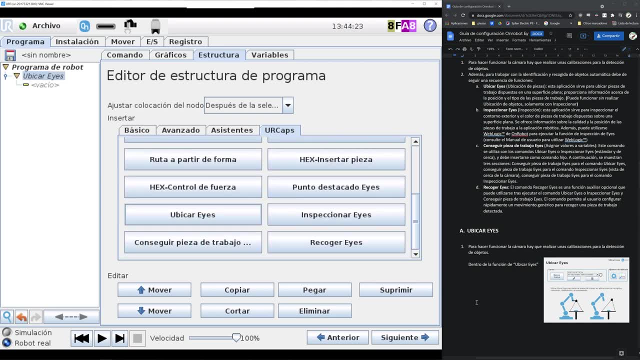 Here we will add a structure already premade by our own robot. We will start off with locate eyes And inside eyes, locate eyes. Inside eyes, locate tree. we add eyes, get work piece And inside this tree we add eyes, pick. So, going back to eyes locate, we will have to add a working area. 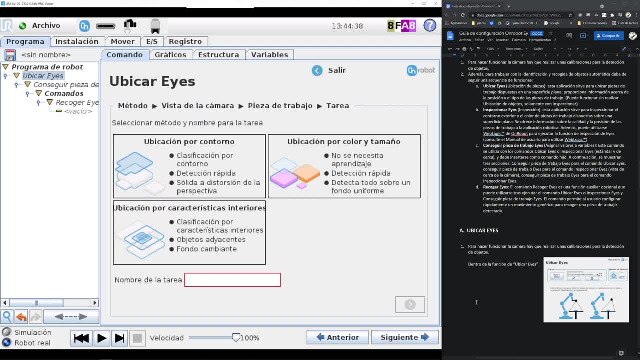 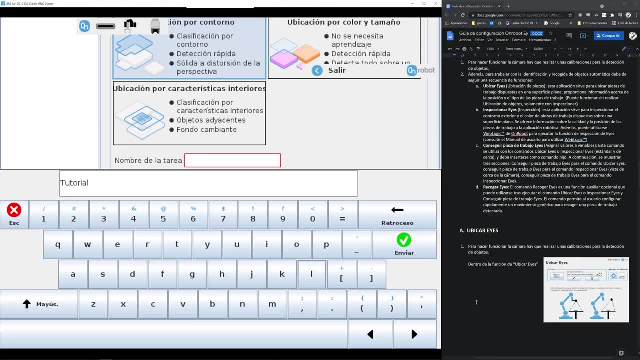 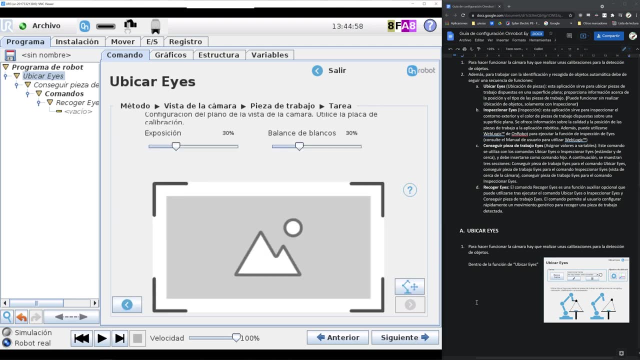 So we start a new task. We can detect objects by contour, color and size or interior designs. Let's start with contours. As you can see, we don't have any area preselected, So we will add an area Here. we can see it's the end of the R conveyor build. 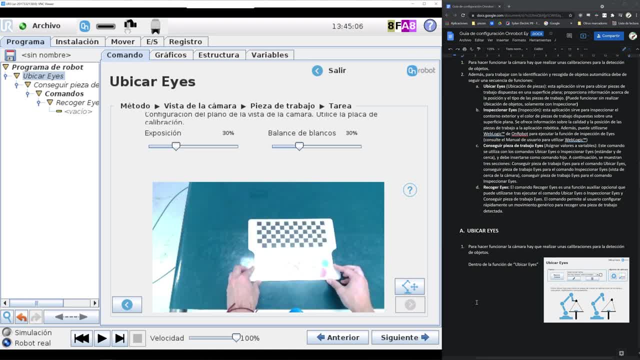 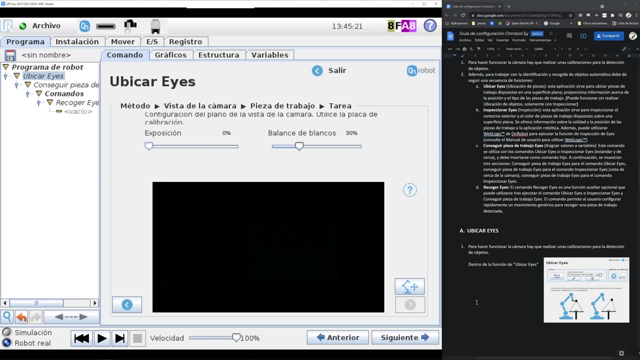 And we have the calibration tool For this. to be able to work and know the distances, You will have to see the green dots in between the white boxes and the black squares. As you can see, you can play a bit with the exposure to see how much light your camera needs. 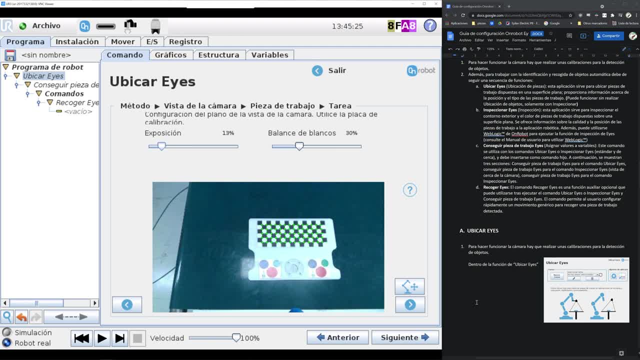 Too much exposure, it's not good, So we select around Between 10 and 30%, depending on the brightness in the room. You need to avoid reflections as much as you can, And colors should reflect or relate to you as much as you can. 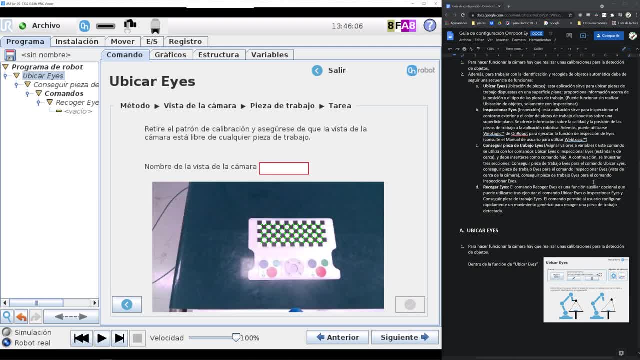 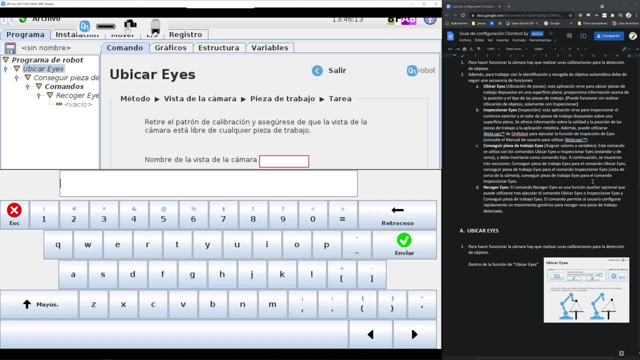 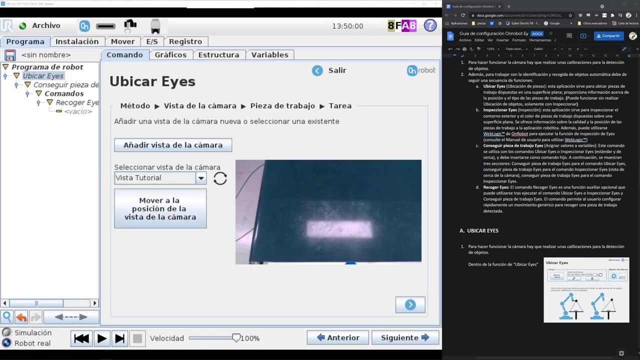 Once done that, you can select next and then get rid of the calibration tool, So you can select the area where the camera will be working on. Now we have the area of the background That the camera will be comparing the objects with And, as you can see, we have one reflection. 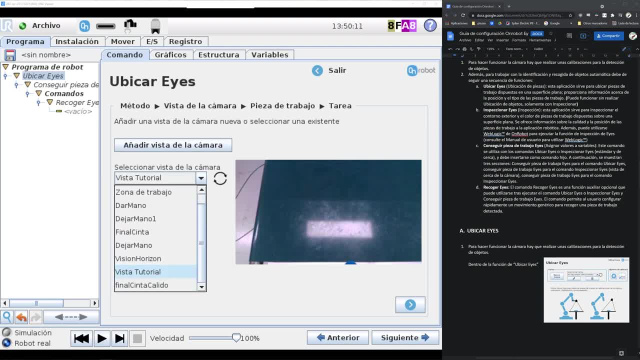 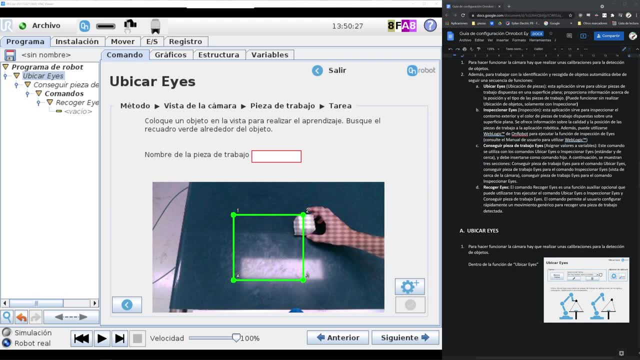 So we will try to avoid that when we are training objects to detect. So we click next and we can see add work piece. We click on that and we see an area where the camera will focus on. In this tutorial, we will use this white cube. 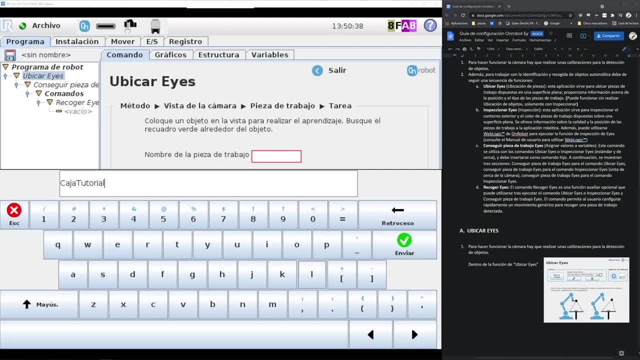 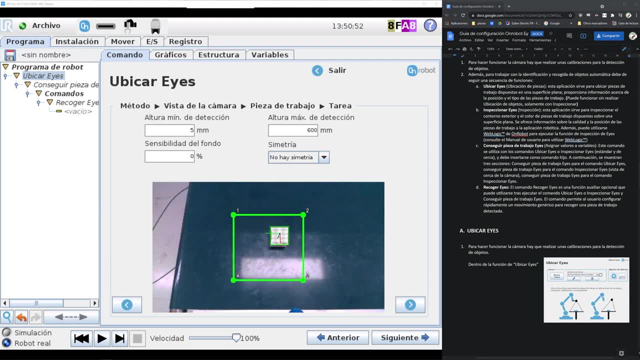 And, as you can see, it detected the contour quite well, So we won't change any configurations. And it didn't detect the reflection, So we will leave that working area as it is. As you can see, you can also play with the height of the object. 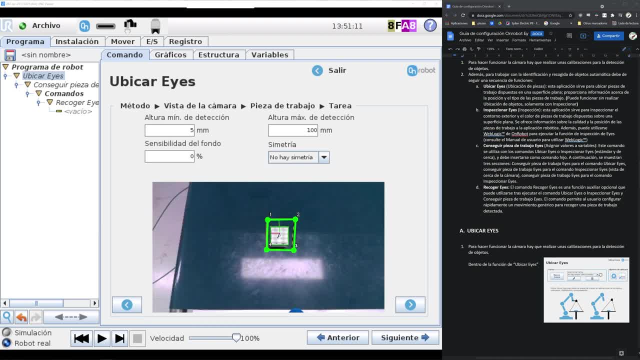 Because once you train with the checkers pattern, It will detect also the distance between the camera to the object. And to make the camera work better, we will make the area smaller. To go next, you have to have a green rectangle over the object that you are training. 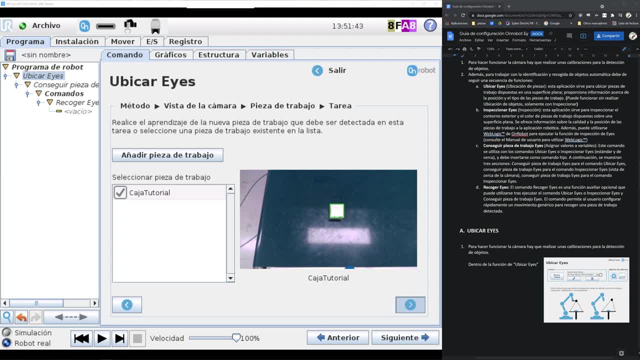 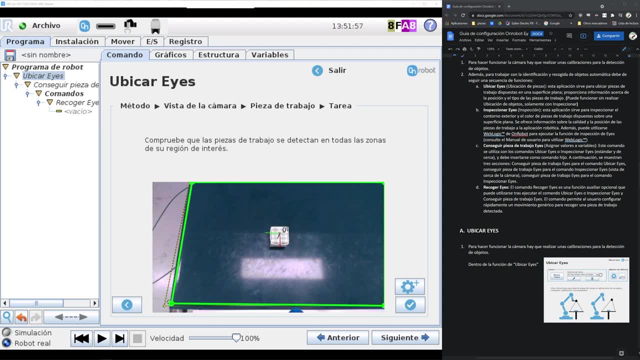 In this case, you can see the white box. Well, the cube, It's selected green. This is the area where the camera will be working on, So we select all the conveyor belt. If you click on the cog, you can change other parameters. 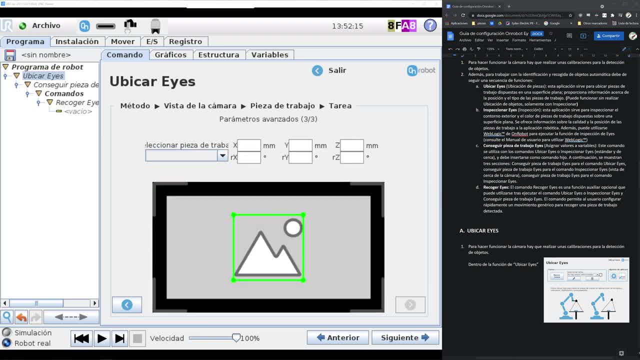 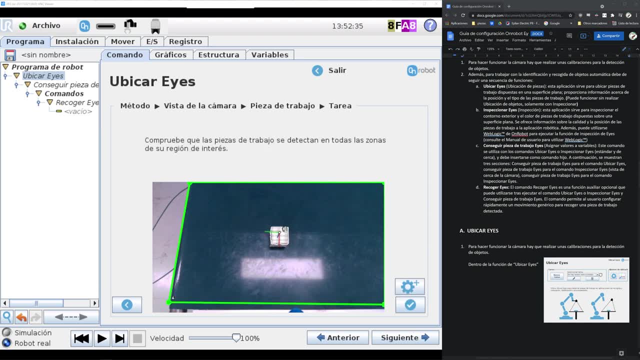 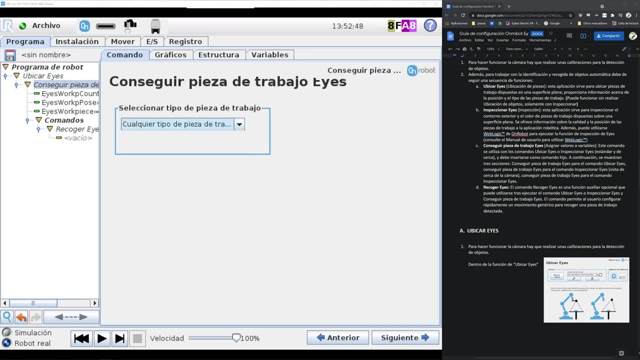 Like where the tool will be getting the object from, Like from top to bottom or from left to right. And then also you can change a bit of the TCP So it doesn't squish the object. Maybe it has a detector So you can actually manually select that. 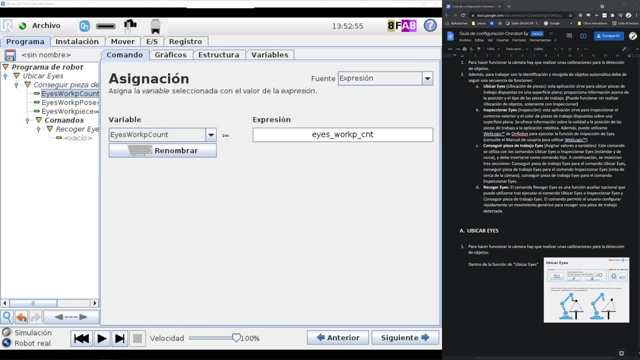 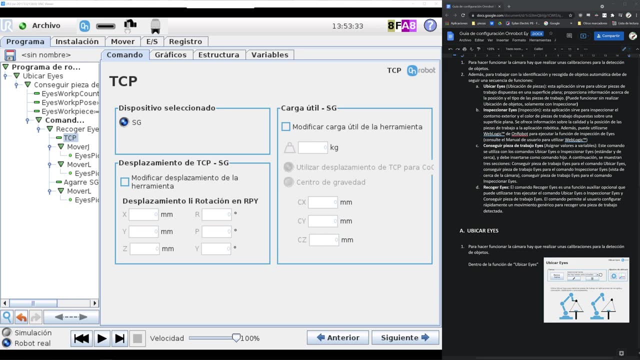 So inside Ice Workpiece we select the object that we just trained And then we can see we can obtain three types of variables: How many objects of the same type, The position of the objects And the type of the piece. Inside Ice Pick we select the generic code. 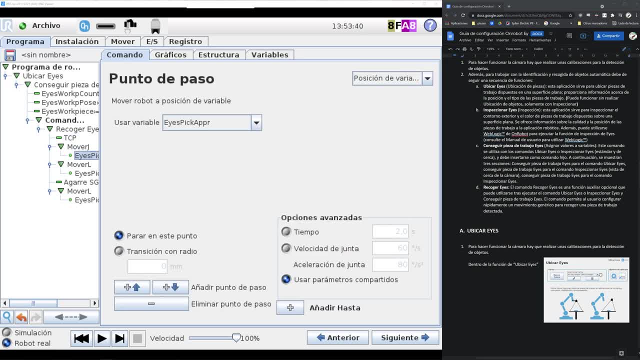 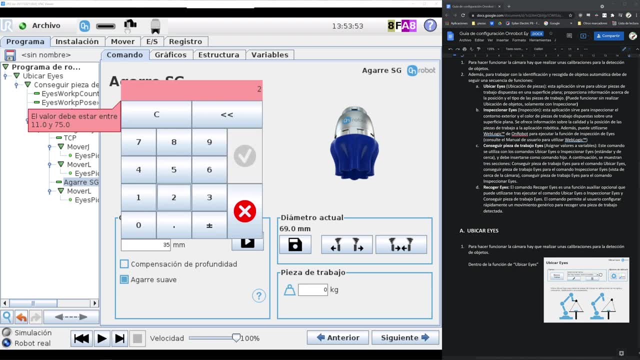 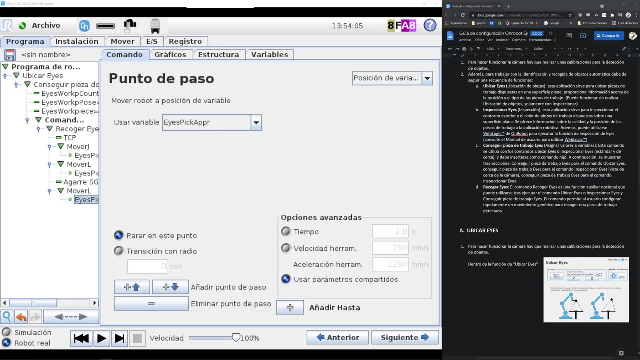 And then there is some predetermined moves that are already automated. In our case, the robot detects very well The cube, So there is no need to change any configuration, Only the diameter of the soft gripper And, as you can see, we change that. 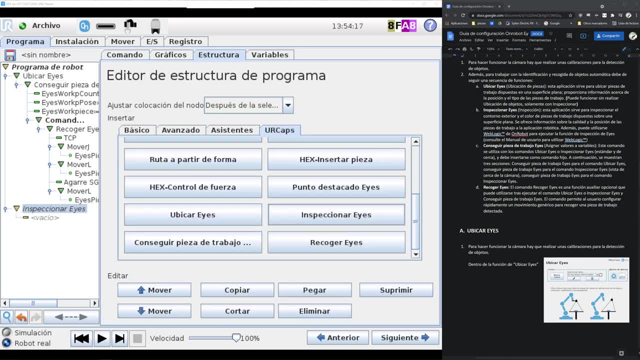 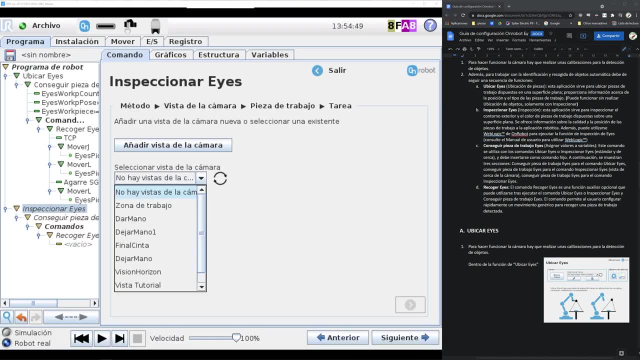 As I was saying before, On-road has three different types of functions. One is Ice Locate, The other one is Ice Inspect And the last one is Ice Landmark. The difference between the first and the second one Are the variables provided after the object recognition. 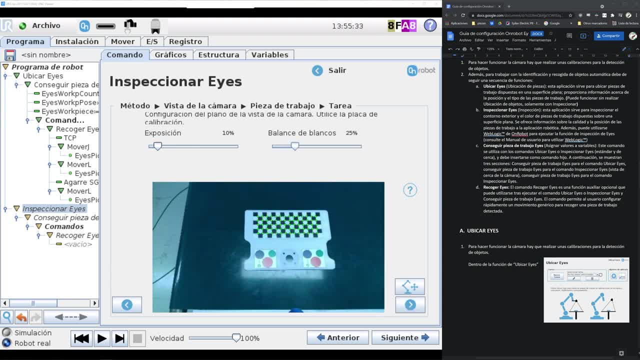 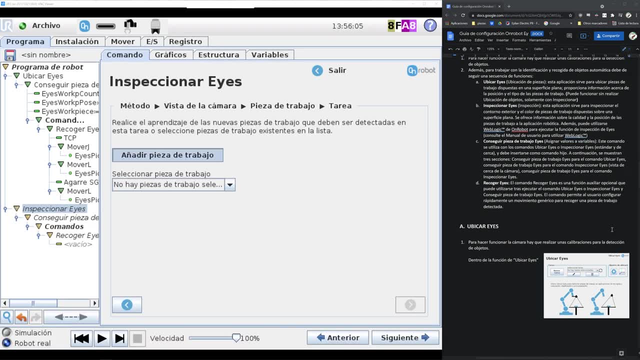 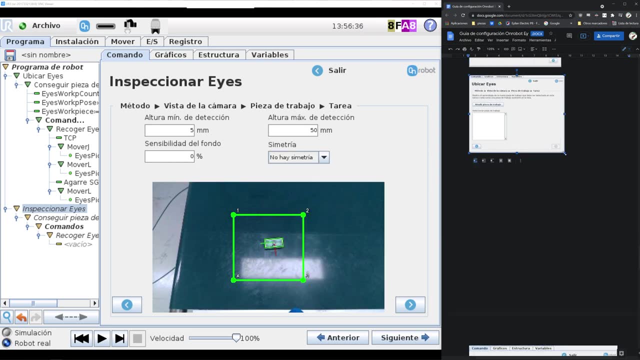 As I said before, Ice Location gives you three variables Providing the location, The number of objects And the type of the object. Ice Inspection, on the contrary, Only gives the quality and position. As the name suggests, It's more focused on quality control. 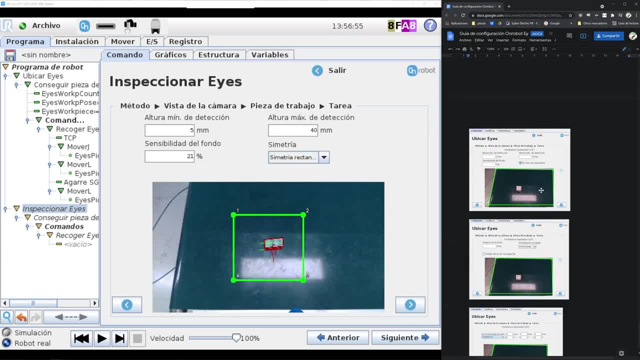 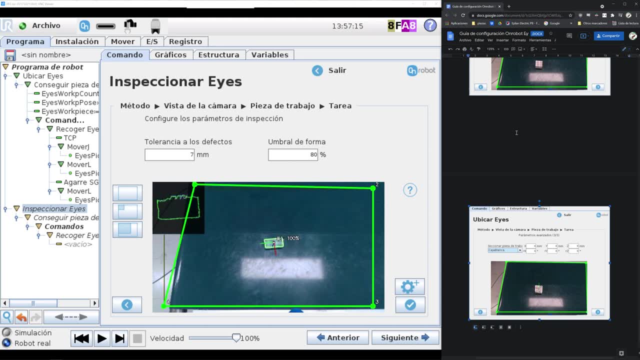 And last but not least, Ice Landmark Is a function used to create applications Where the robot and the part of its workspace Are not fixed to each other. Here we can see an example of Ice Inspect. It's comparing the contour of the object. 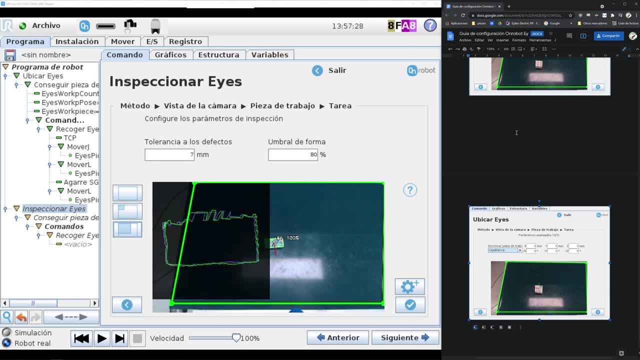 That it's been detected With the object that has been trained. The training is the same as Ice Location, But the difference here is that You can select the defect tolerance And the shape threshold After finishing the training. As you can see, 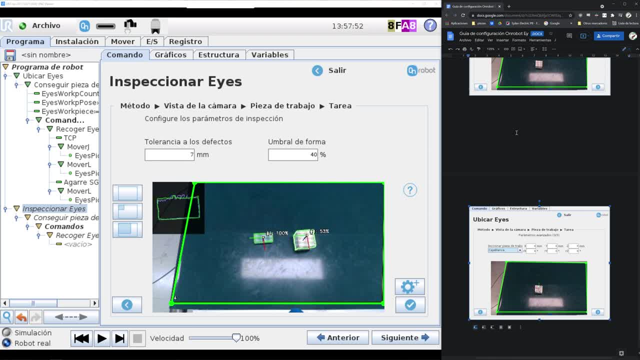 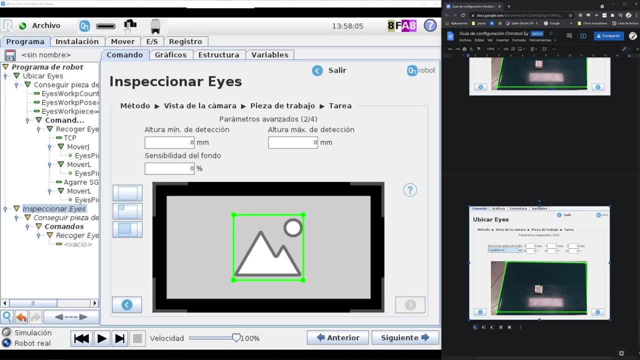 There's a hundred percent coincidence With the object that has been trained, But a fifty percent with the cube That we trained before. If we bring down the threshold, It will allow the cube also To be selected and picked. The command tree. 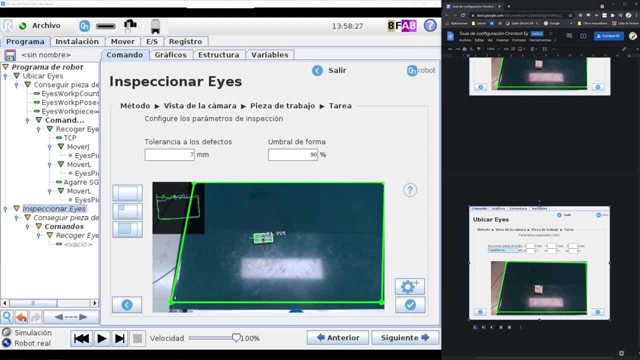 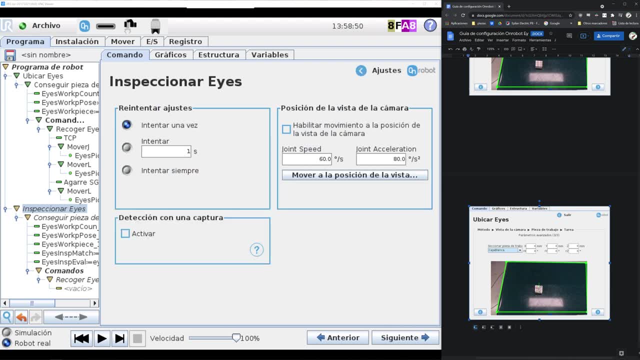 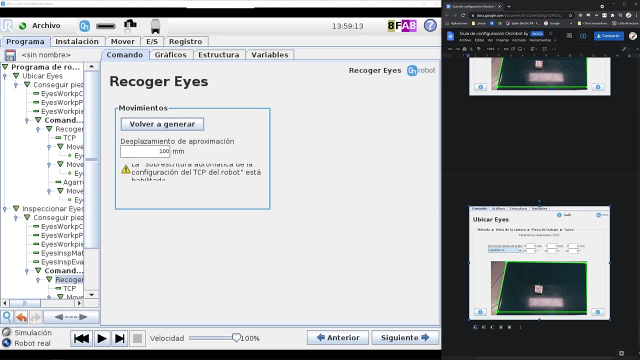 Is just basically the same. as you can see, Ice Locate and Ice Inspect Are both the same pattern. You first choose Which function you want to use, Then Ice Get Workpiece And then inside nested Ice Pick. Like I said previously, 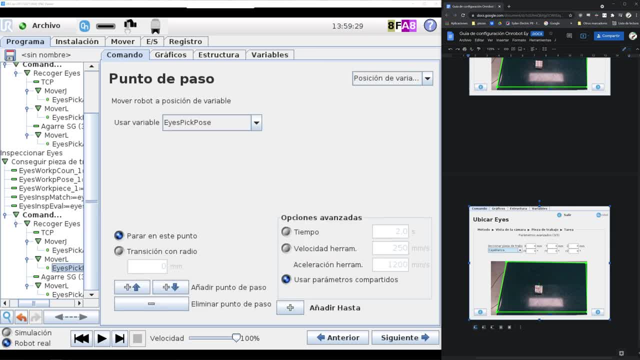 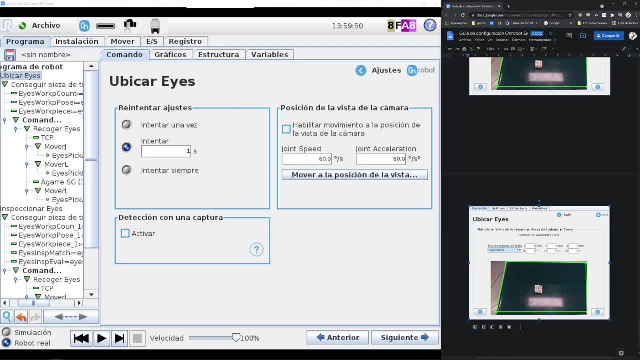 If you need to modify the TCP Or the movement, From where, The direction, where you want to pick the object, Here are the options. But since it's like A rectangle, It's also No problem. And The ice? 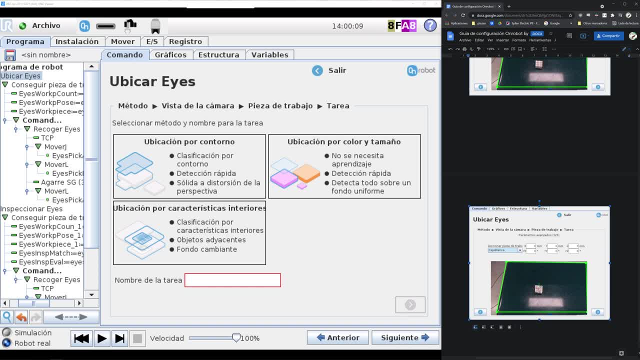 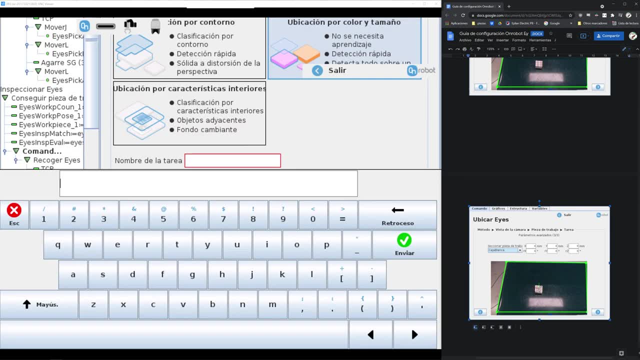 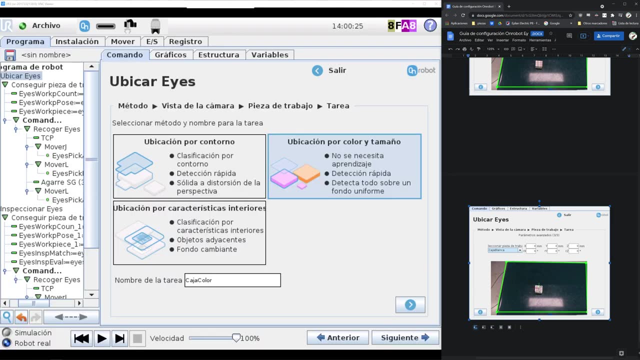 Can see the distance, So It gets the Object quite well. This is another example of Object recognition by Color and size. So we select the option. We put a name Of the piece So we can Create another working area. 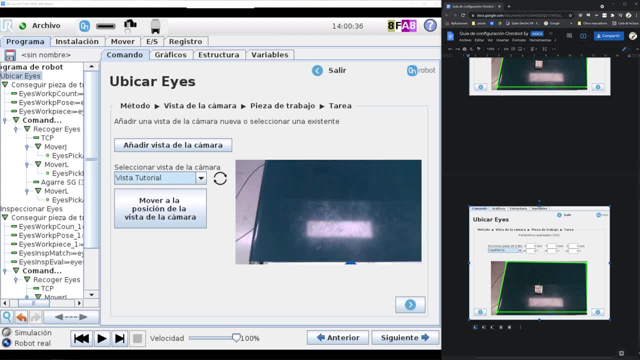 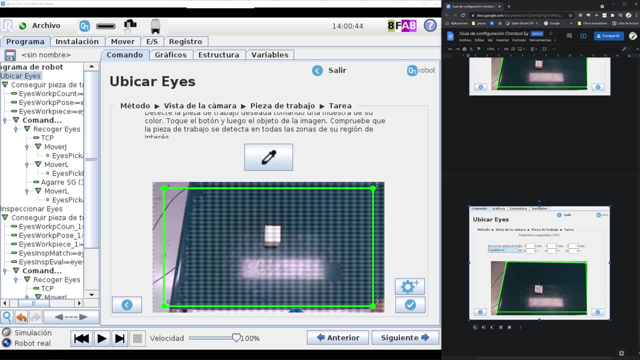 But we choose One we previously used. So Tutorial View, And here You can see the Classic icon To select the color. Right now it's Detecting everything. So, As you can see, We Create an area. 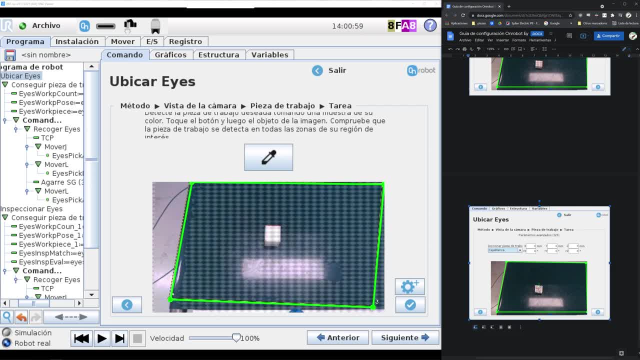 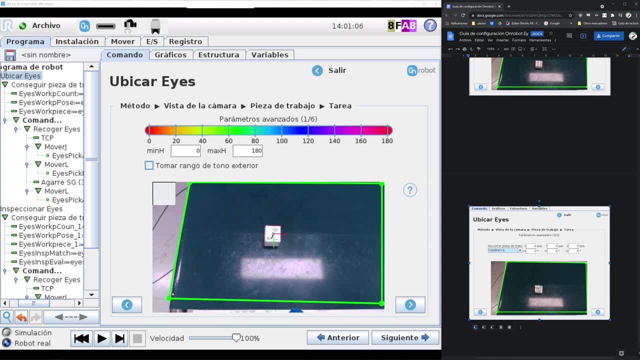 Of the conveyor belt And we Select the Box And Later on You can tune The parameters. But Since it's detecting The box Quite well, We'll just leave it Like that. I'll show you.